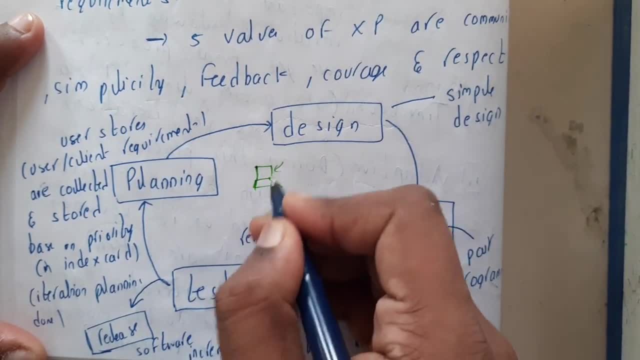 project. So you are making a project. So you are making a project. So you are making a web application to download some files from online. So you made a website for that. So for that, initially you don't need any login page or logout page, right Or registration. 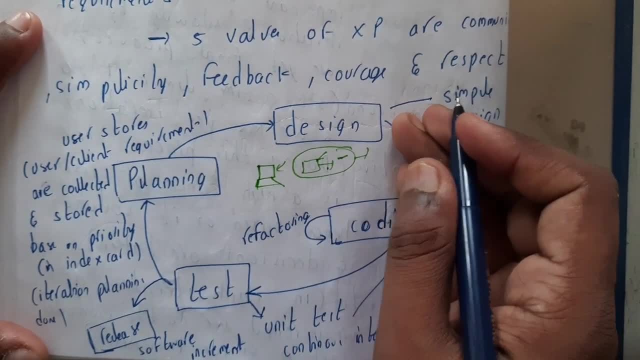 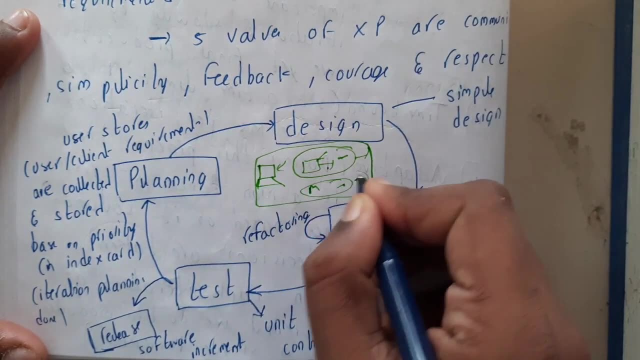 page. So these things will be of no priority or of less priority, Whereas the management of downloads and all those things will be of high priority. So, based on the priorities, you'll be separating them in planning only. Okay, so based on that, you will be starting. 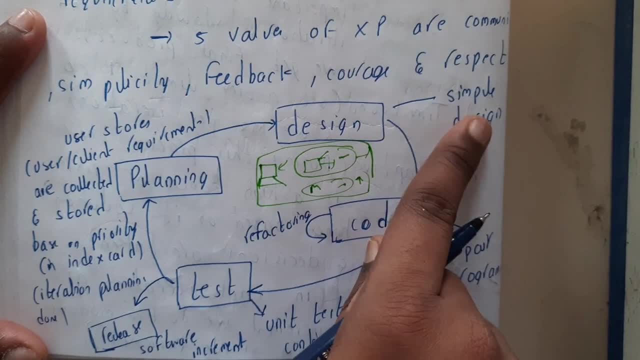 your design. So here we will be doing some simple design tactics, and we'll be doing it, right, Okay, And the next step will be coding. So here we will be doing some simple design tactics and we'll be doing it, right, Okay, And the next step will be coding In coding. 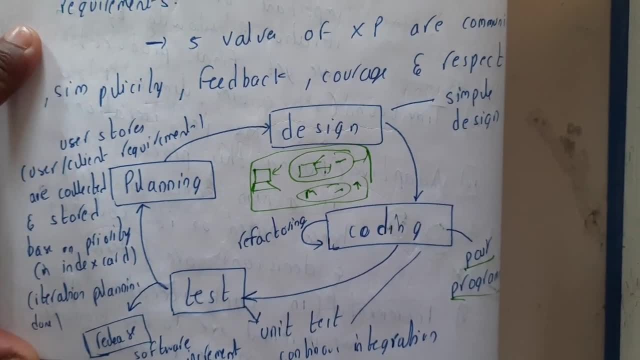 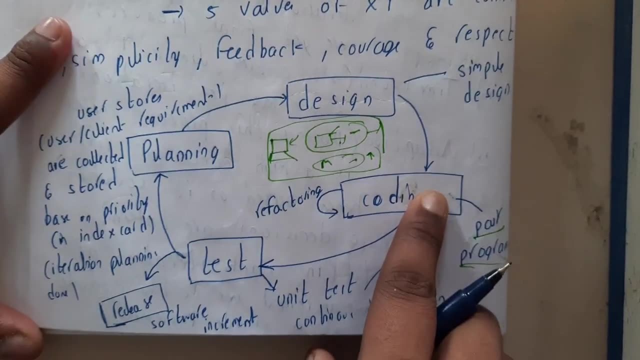 we will be following a special practice which is called as peer programming. Okay, so we'll be discussing about that, guys, Don't worry. And in coding only, we'll be doing refactoring. This is also we'll be discussing, Don't worry, And once the coding is done perfectly, we'll 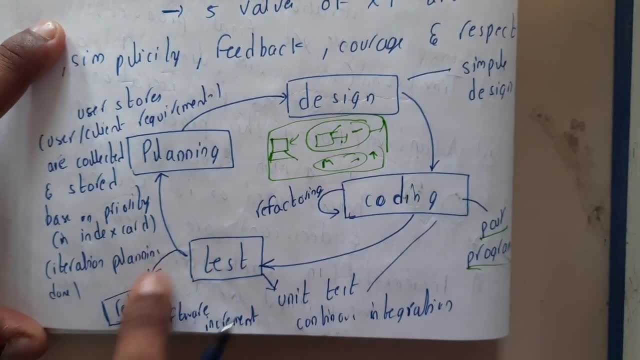 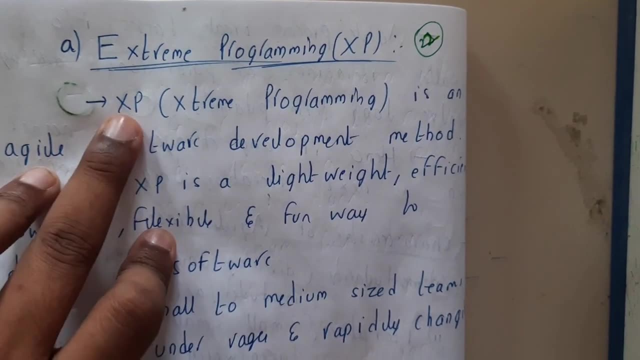 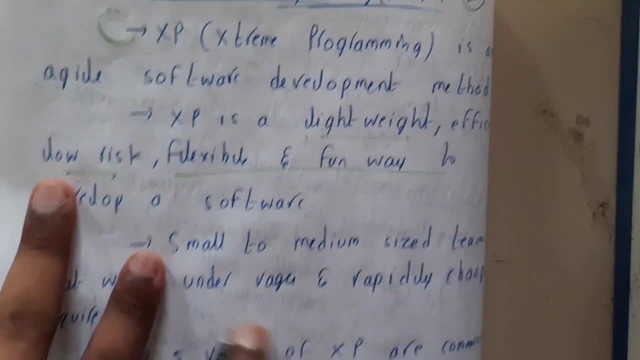 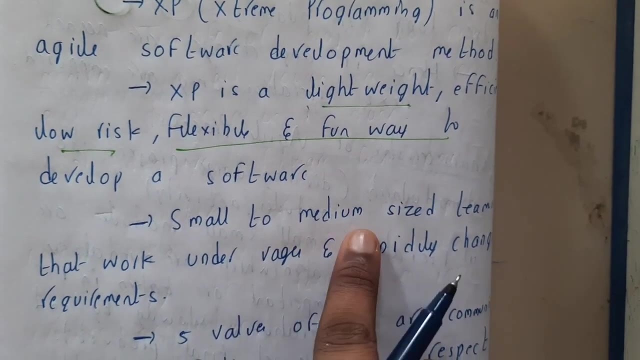 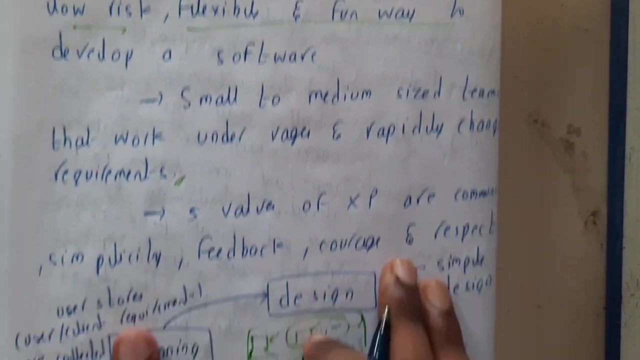 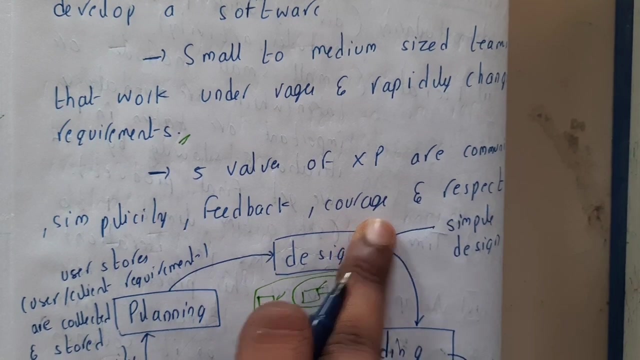 and fun way to develop a software guys. Okay. So basically extreme processing will work on smaller or medium scale teams and projects. So small to medium sized teams that work under wages and rapidly changing requirements are best for this extreme programming. So we are having five basic steps. Okay, basically we can say that: communication, simplicity, feedback, 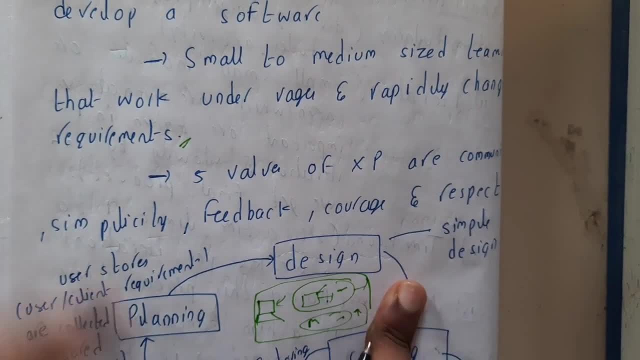 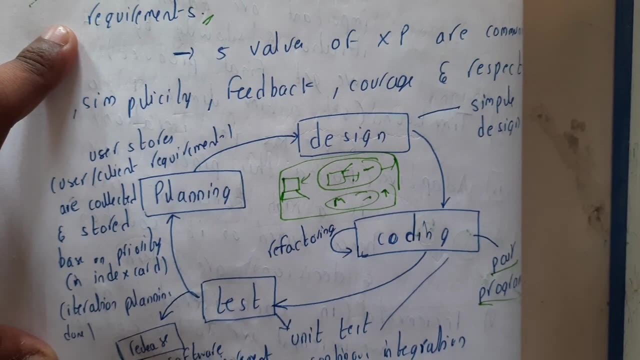 courage and respect. So we'll be saying in that way, but in the diagram we'll be just representing them in the normal way. only guys. so we'll be starting with planning, designing, coding, testing and release. so basically planning. i told you previously also so user, so we will be collecting the requirements. 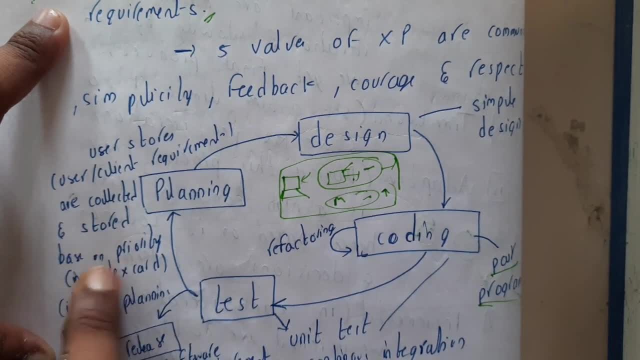 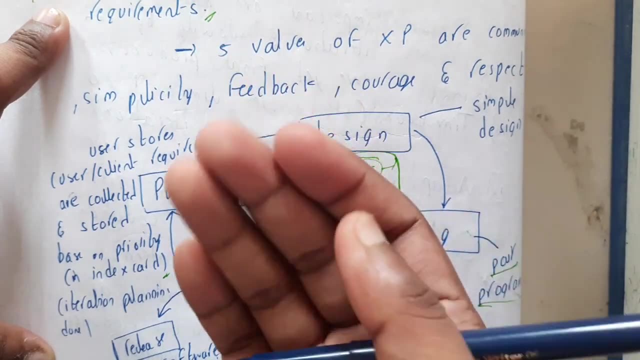 so we will be storing the requirements according to their priority. so priority those things. we will be calling it as index card, so assume that it is as a visiting card on which you are writing the priority number and what is the requirement. so those are nothing but the index card, okay. 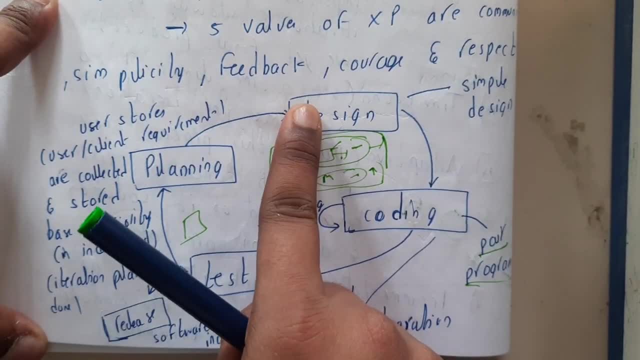 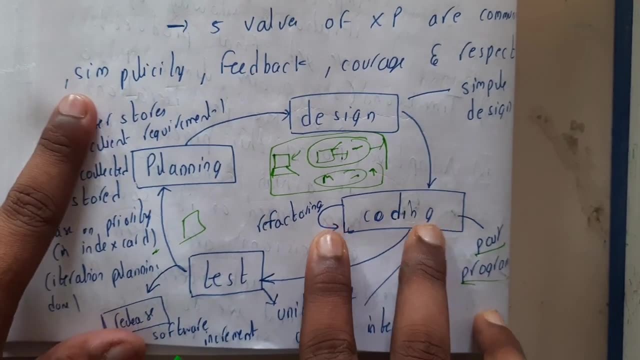 so, once it is done, the planning is done, you will be going to designing. so, in design, you will be making the high-end design for the particular plan that you have understood. okay, then you will be moving on to coding. so, guys, if you want theory about planning, decision designing, coding, testing, 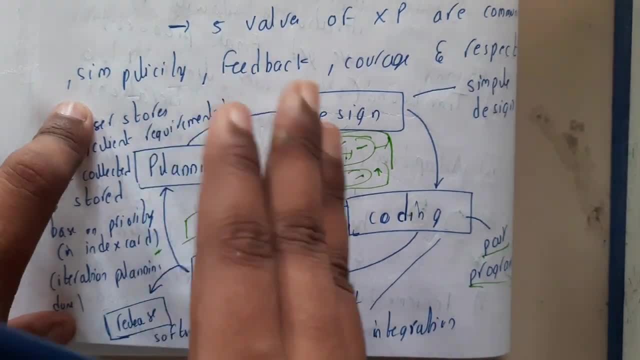 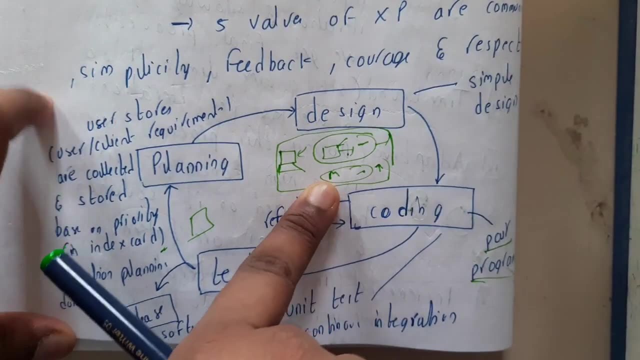 and release. please go through our previous lectures, guys in sdlc. from sdlc, we are discussing the same topics, so you can check the notes. or you can get the notes from sdlc and waterfall model. okay, okay, so from in design, you'll be getting the output as a particular neat design. 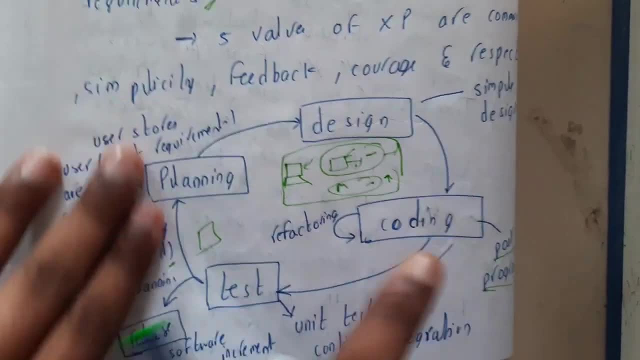 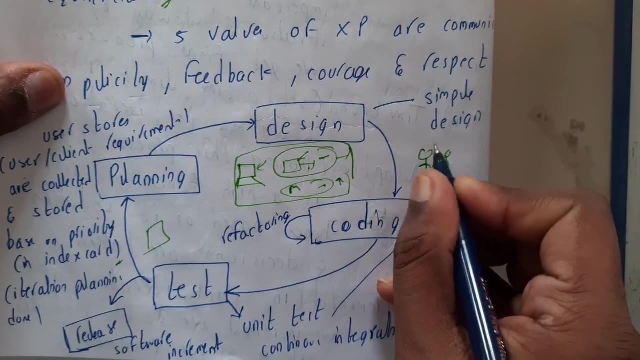 so you can check the notes or you can get the notes from sdlc and waterfall model. okay, okay. so, coding in coding, we are having pair programming. okay, guys, if possible, sometime, someday, you try it guys. so, basically, you bring your friend and you you code in front of him. he'll be just sitting. 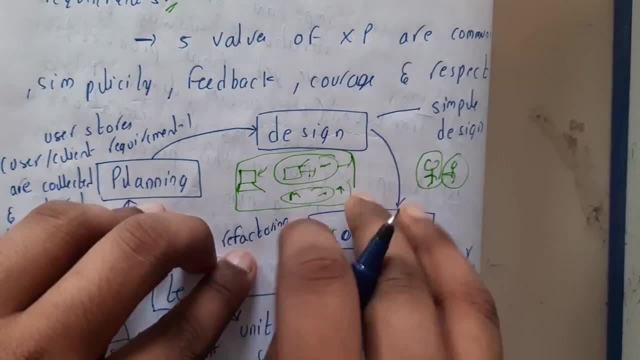 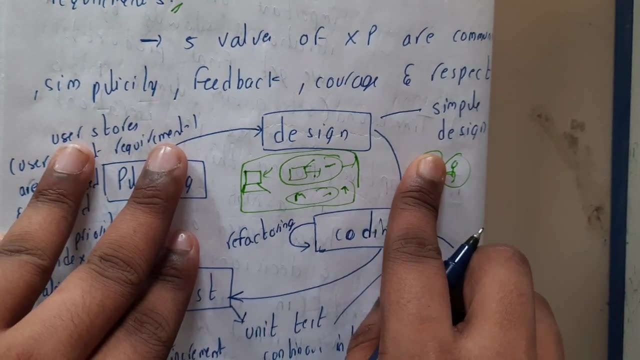 there beside you and he will be observing how you are coding, like: what are the types you are coding, is there any missing or if you are doing anything wrong. he'll be identifying him, identifying them, and you will be writing sorry, you will be writing the code and he will be. 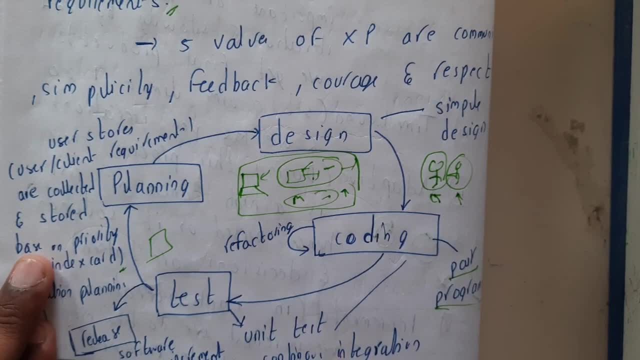 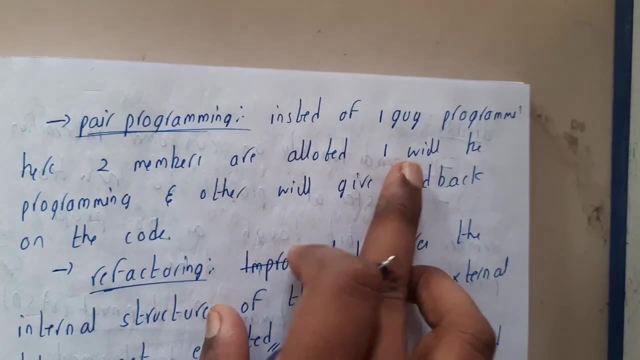 checking the code and he will be testing the code, guys, okay, to be clear. okay, so that is nothing but pair programming, if you want. in words, pair programming instead of one guy programming. here, two members are allotted: one will be programming and another will be giving the feedback on the code. so basically he'll be saying that, okay, that test case will fail, bro, like that. 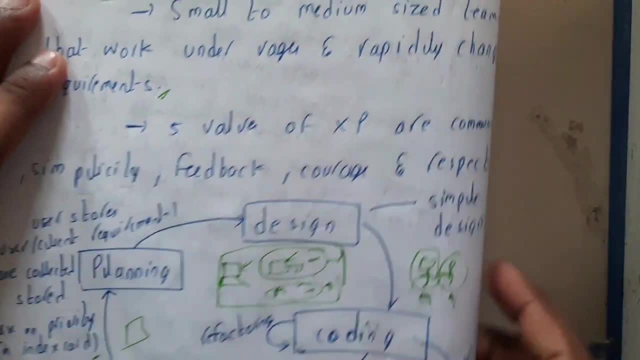 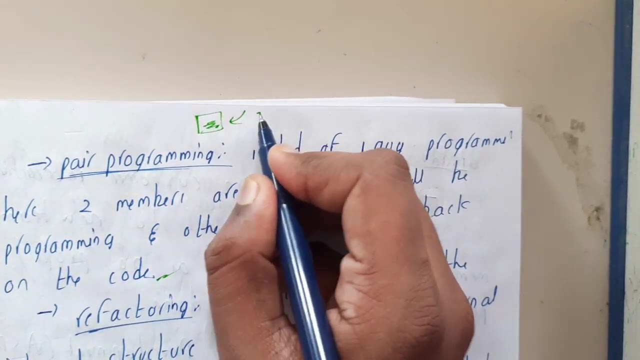 he'll be giving you information about those things. okay, refactoring, refactoring. it is really simple, guys. it is just improvement of the code. so, basically, if you wrote the code in a bit lengthy way now using refactoring, you will be making it condensed, or you will be reducing it, or you will. 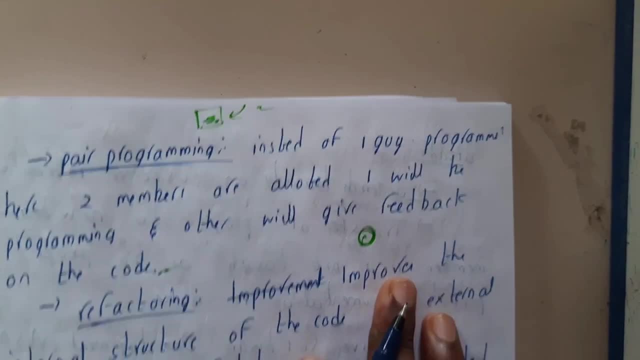 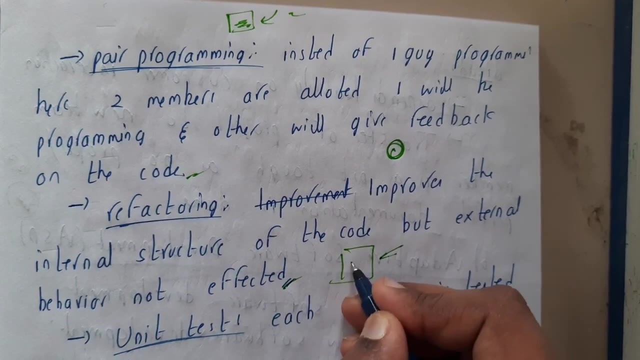 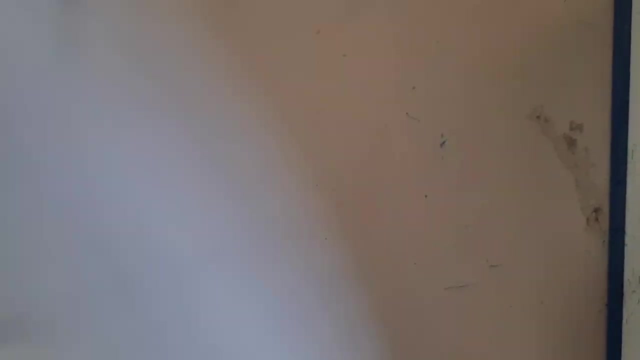 be removing the unwanted things. so refactoring, refactoring, refactoring, refactoring, refactoring improves the internal structure of the code, but external behavior will not be affected. so the code will work exactly the same, but the internal structure, like the for loops, brackets and everything will be set at properly. okay, so once coding is done, you will be moving on to testing. 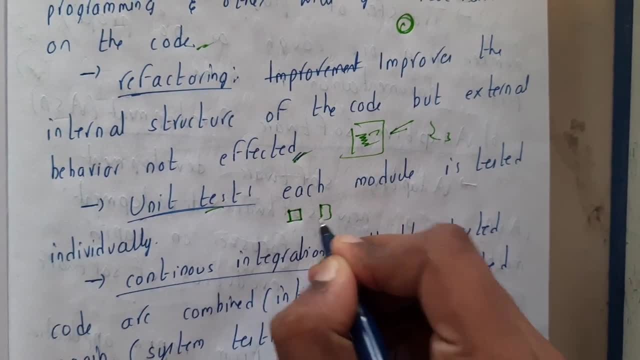 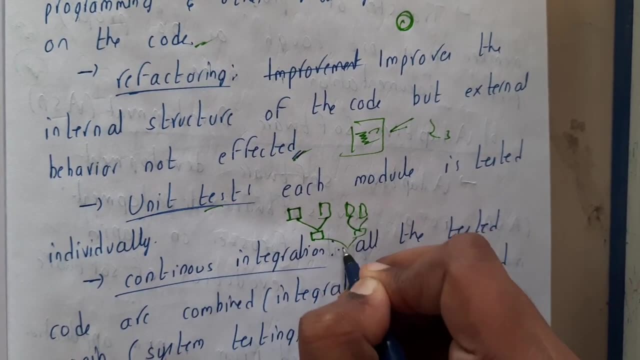 so i hope everyone knows what is unit testing. so each and every small, small module will be tested individually. guys, and integration testing is nothing but combining these two and you'll be testing the modules. at the end. you'll be combining these both and testing the final module, so that is. 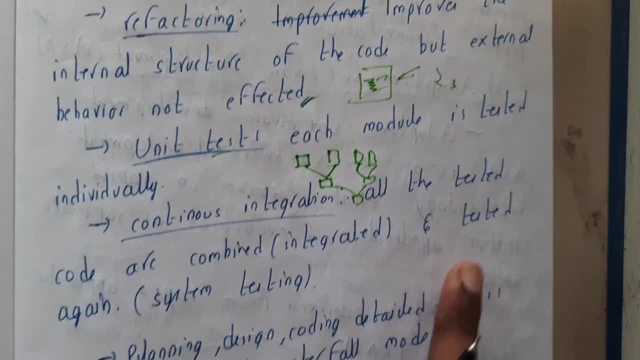 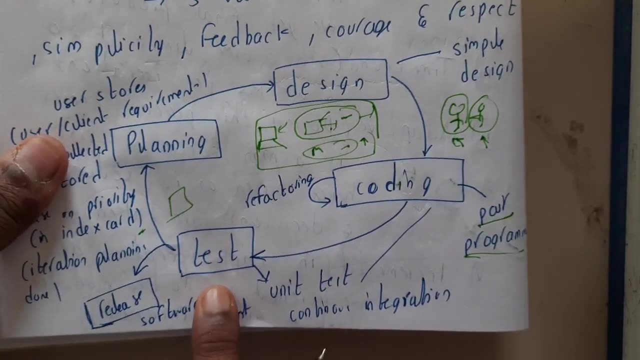 nothing but integration. so all the tested codes are combined and you will be testing the modules combined, integrated and tested again and again. that is nothing. that is also called a system testing guys, okay, okay. so now, at the end, we will be releasing the software to the globally. okay that. 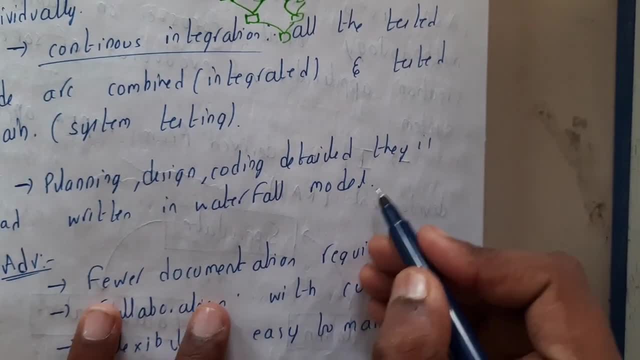 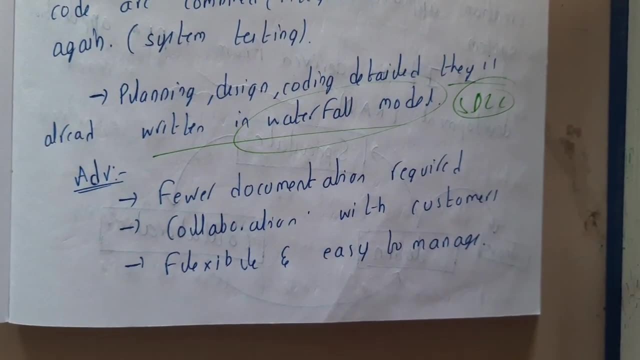 is nothing but one software increment has been done. okay, so, guys, you can find the notes as we have written in sdlc and in waterfall model. okay, so the main advantages of this model is that we will not be having much about documentation. is nothing required, guys, because we are maintaining. 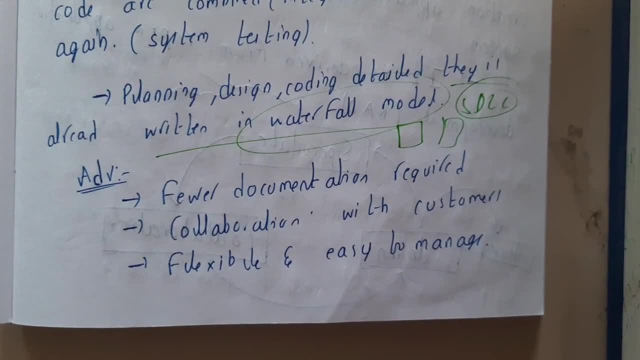 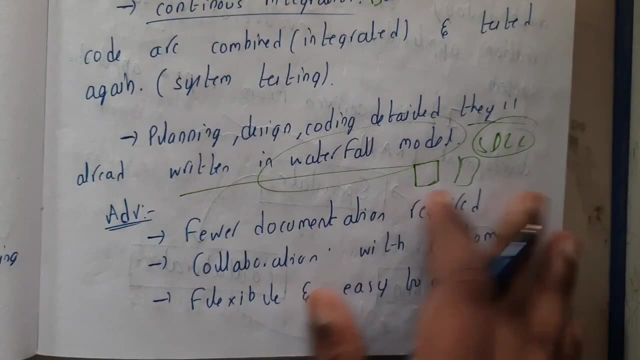 everything in the requirement, analysis and planning only. we are doing everything right, so we are creating those cards, and on the cards, only index cards. right, just give me a second. yes, index cards. okay, so on index cards only, you are mentioning everything like what are the requirements, what is the priority for it, and everything. so 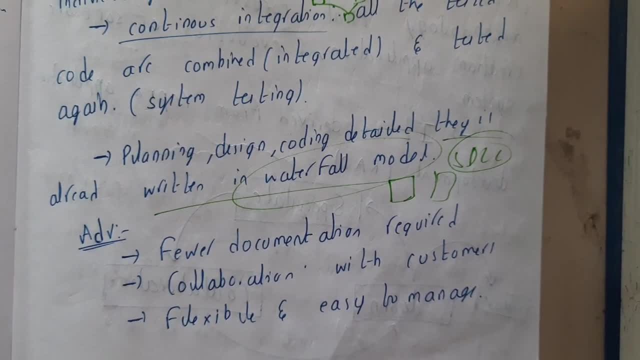 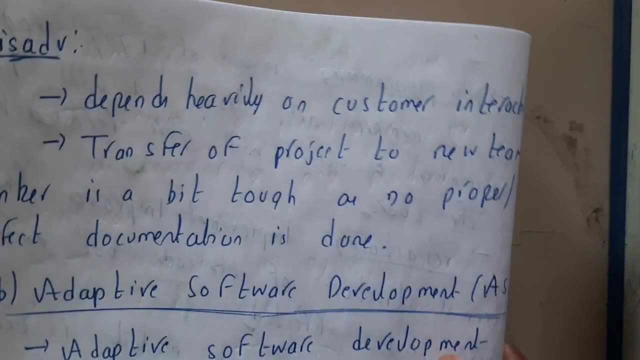 hence, there is no much documentation required while collecting the requirements, and collaboration with customers is high here, yes, flexible and easy to manage: yes, and the major disadvantage is it depends heavily on customer interaction. so, basically, you are getting the inputs from the customer, right. so if the customer is not getting the inputs from the customer right? so if the 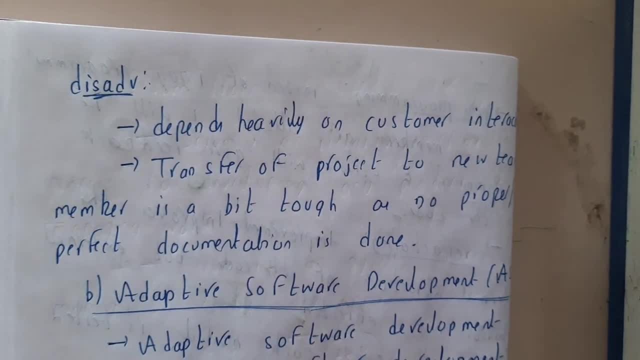 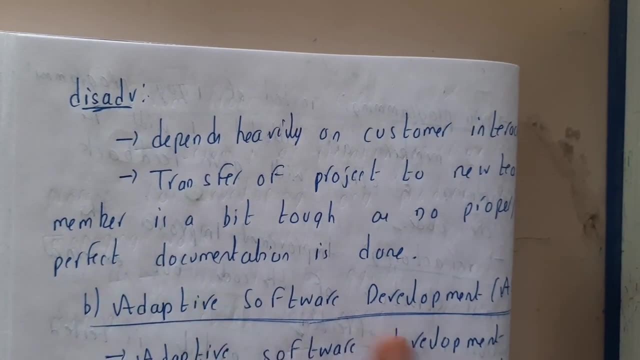 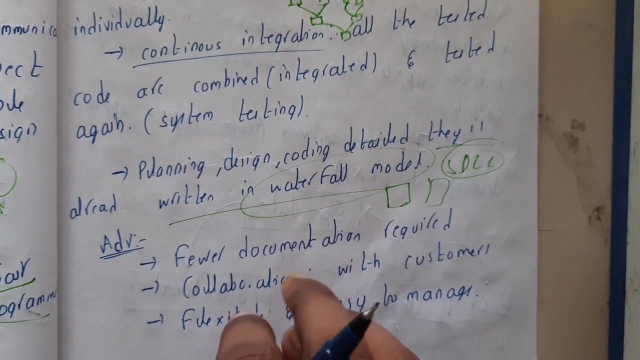 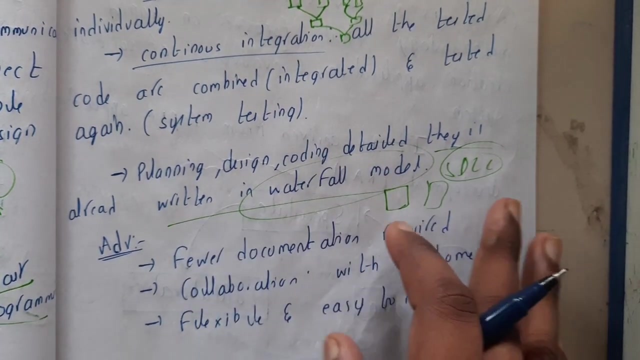 customer is not having clarity or he is not interested in discussing with us, that could be a huge issue, right? yes, transfer of project to a new team member is a bit tough as no proper or perfect documentation is done. so, basically, i told you that we are not having any proper documentation. we are just maintaining the cards. so if you are, if the project team leader or the developer who is working on this project has been sick or due to some technical issue or due to his personal issues, if he resigns or if he changes the job, then there will be a huge issue because he is not having clarity or he is not interested in discussing with us. that could be a huge issue, right? yes, transfer of project to a new team member is a bit tough as no proper or perfect documentation is done. so, basically, i told you that we are not having any proper documentation. we are just maintaining the cards. so, if you are, if the project team leader or the developer who is working on this project has been sick or due to some technical issue or due to his personal issues, if he resigns or if he changes the job, then there will be a 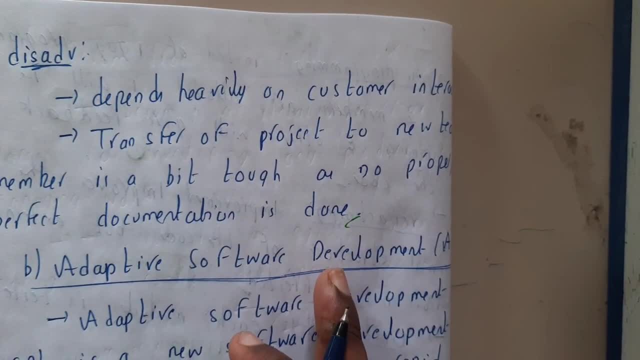 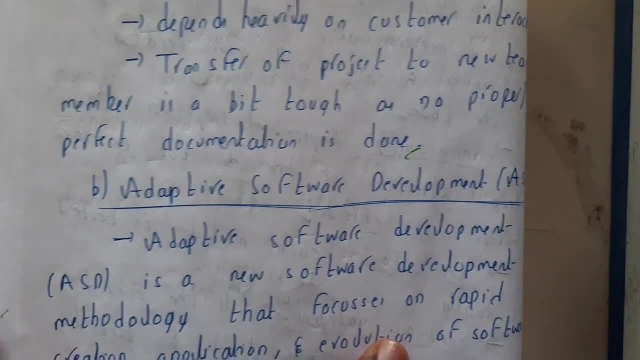 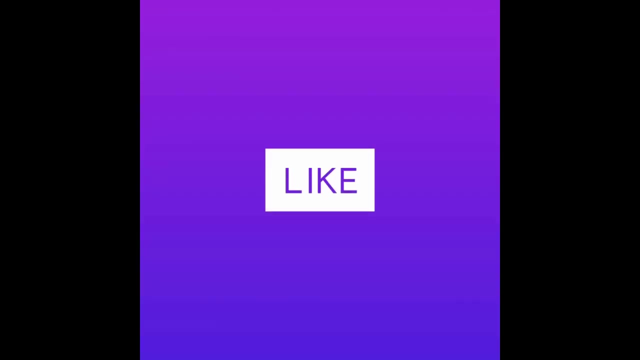 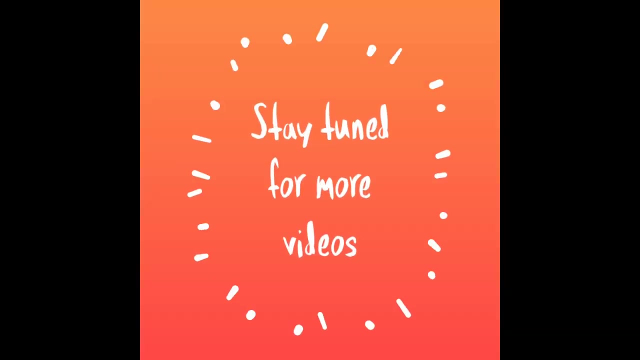 because there is no documentation, no one can continue the project. guys, it will be a huge issue for understanding the code, okay, okay, so i hope everyone got a small idea on this. so in the next lecture we will be going through adaptive software development. okay, so let us meet in the next lecture, thank you. thanks for watching.